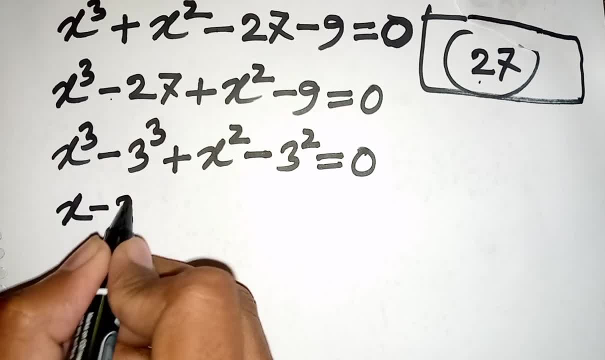 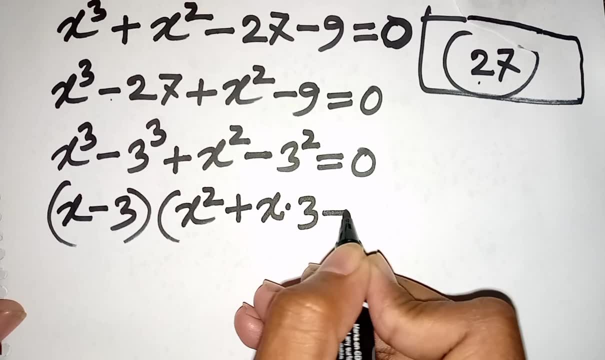 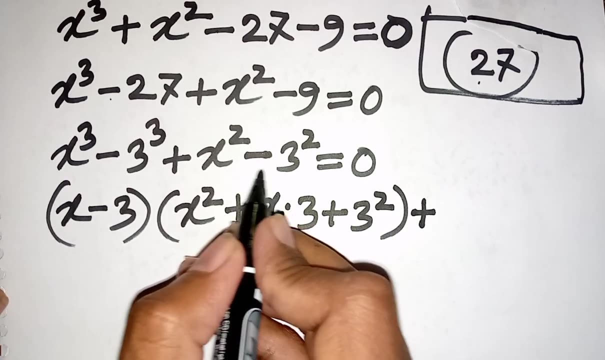 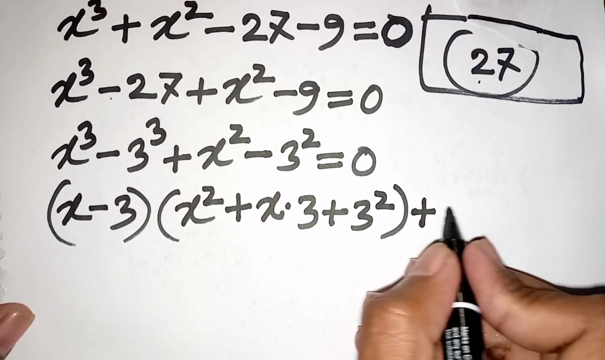 So according to formula, we can write here: x minus 3 times x square, plus x times 3 plus 3 square, then plus. here we can apply the formula of a square minus b square: here a is s x, b is s 3. so according to formula, we can: 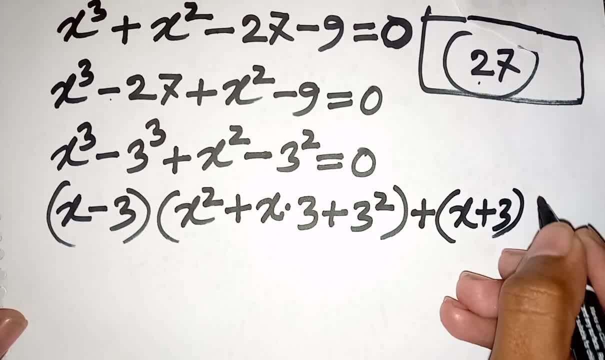 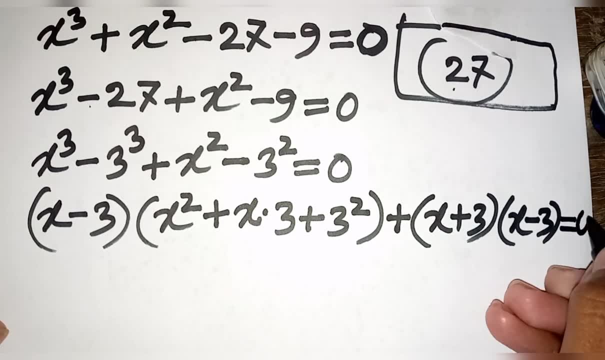 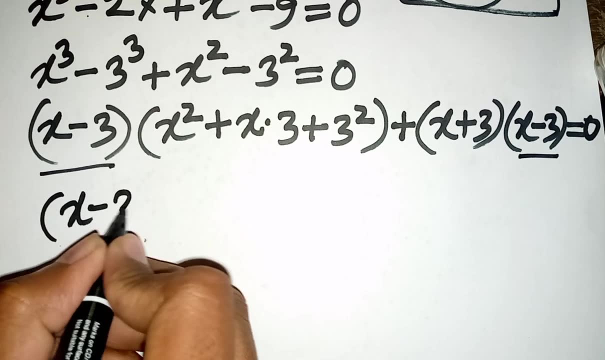 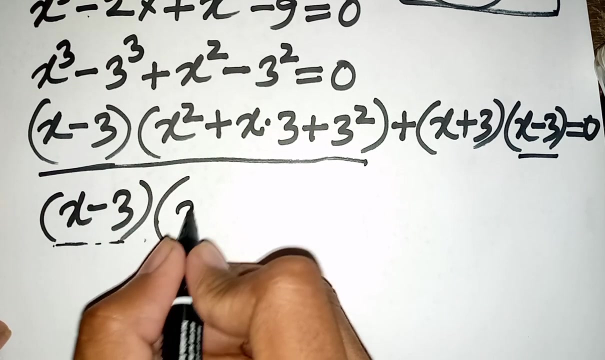 write here: x plus 3 times x minus 3 is equal, is equal to 0. now we see x minus 3. x minus 3 is common, so bracket x minus 3 is out of this bracket. so this divided by this, that means x square. 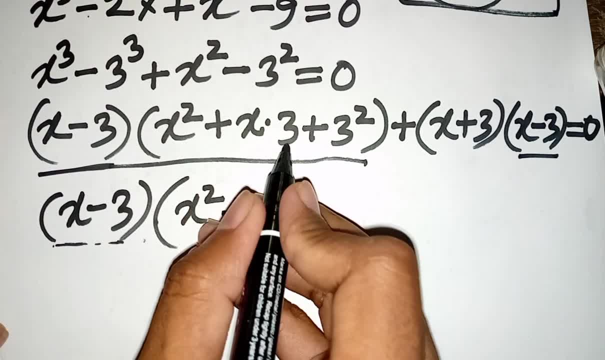 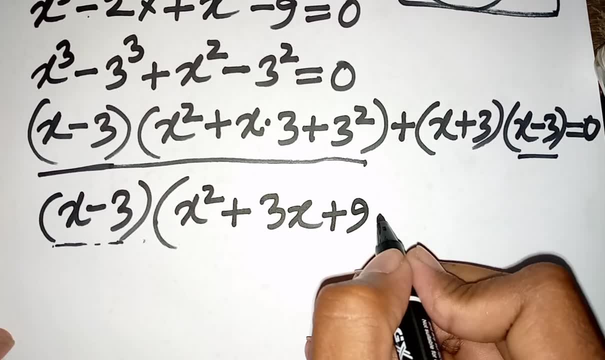 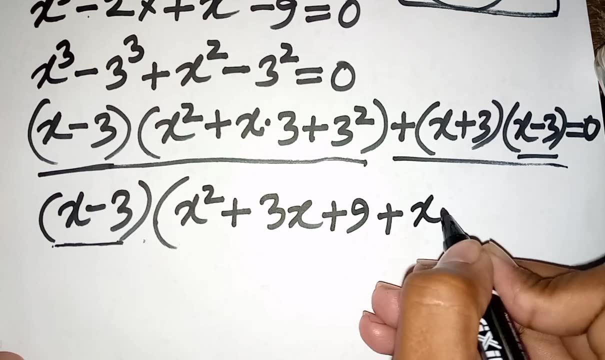 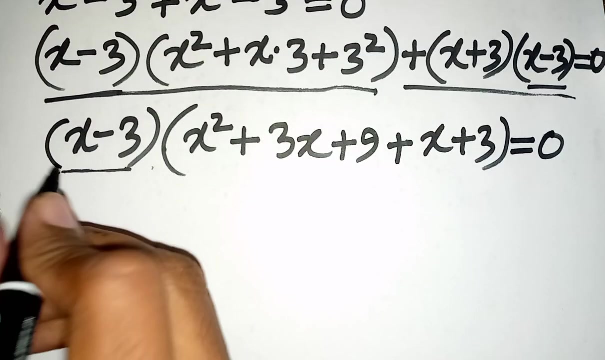 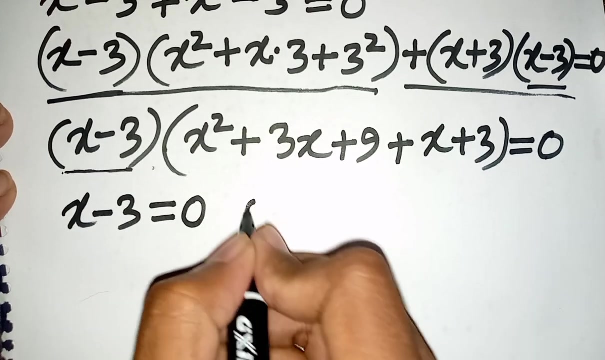 plus x times 3, it will be 3x plus 3 square. that means 9 plus these. divided by this, that means x plus 3, x plus 3 is equal to 0. now now we can write here: x minus 3 is equal to 0 or x square. 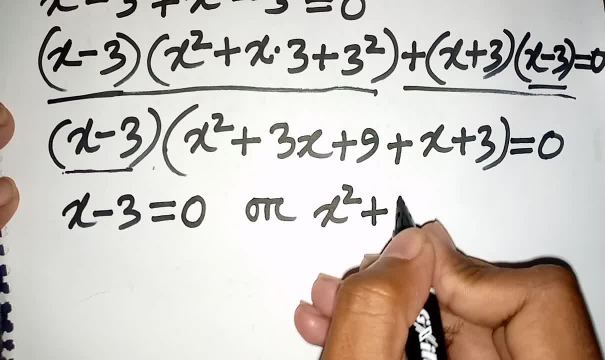 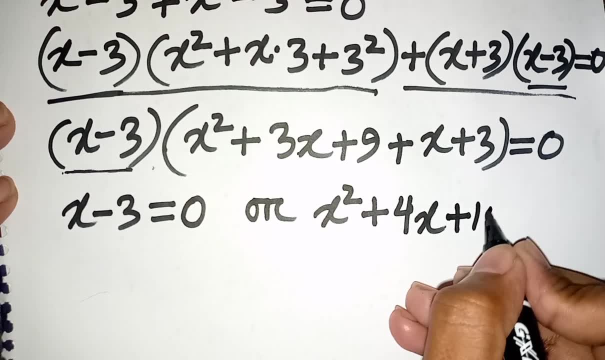 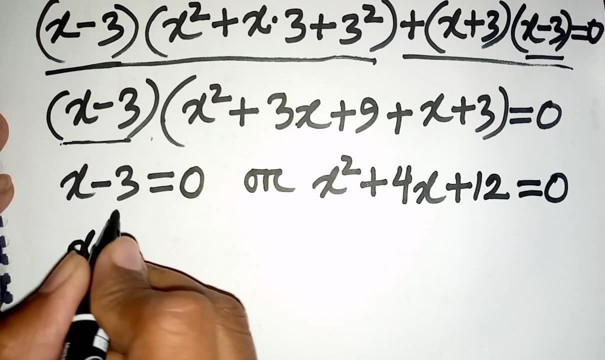 plus 3, x plus x, it will be plus 4, x, then plus 9, plus 9 plus 3, it will be plus 12 is equal to 0. now we can write here: x is equal to minus 3. take to the right side, so this will be plus 3. 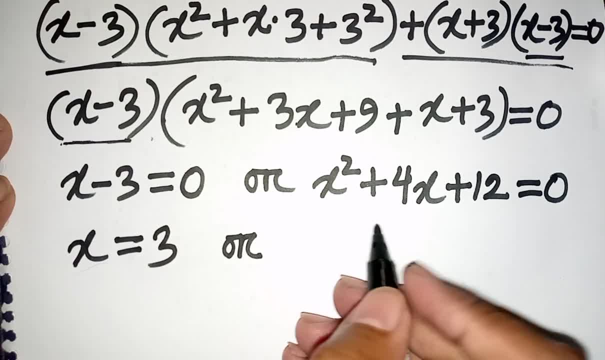 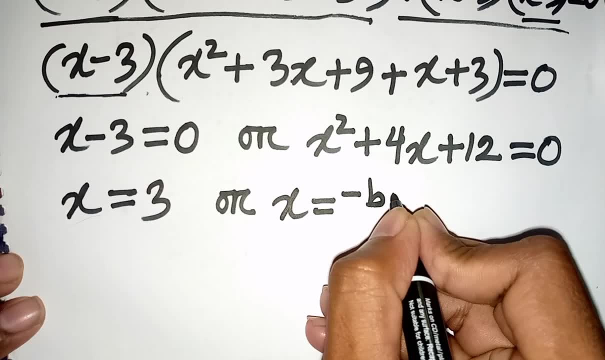 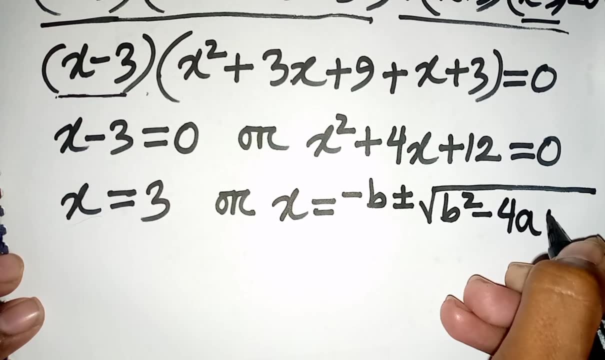 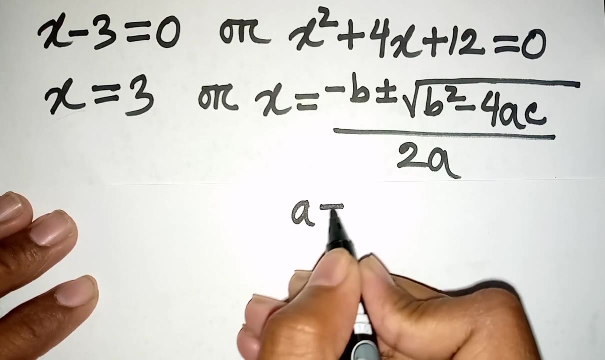 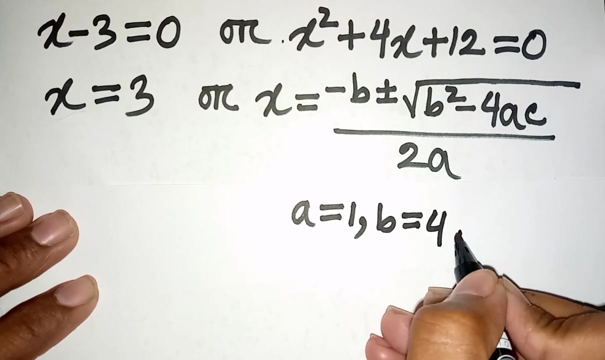 or here we can apply quadratic formula. so we can write here: x is equal to minus b, plus or minus a, square root of b, square minus 4 ac divided by 2a. now here a is s on, b is s 4, c is s 12. 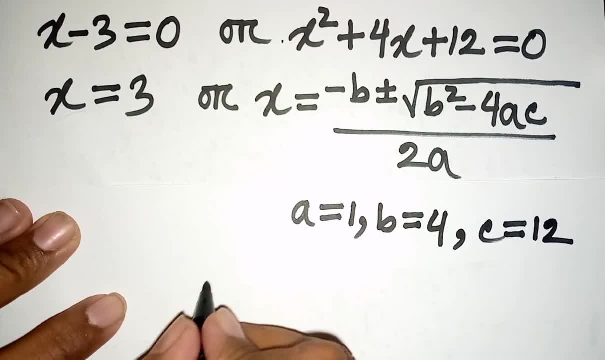 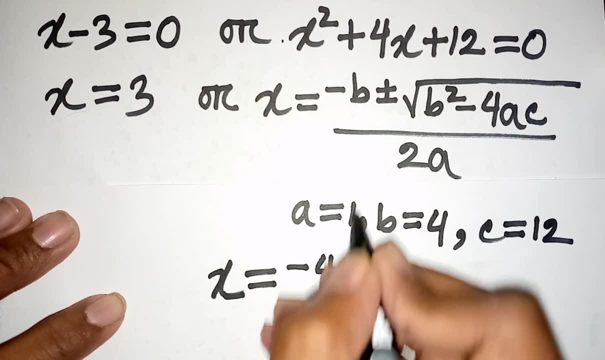 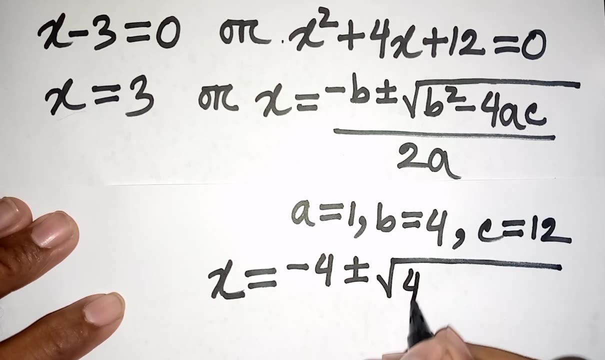 so we can write here: x is equal to minus b. that means 4 plus or minus s. square root of b: a. square, that means 4. square minus 4 times a. that means 1 times C, that means 12. so we get 4 products. because for the product is 4, you need to be square. this is적. 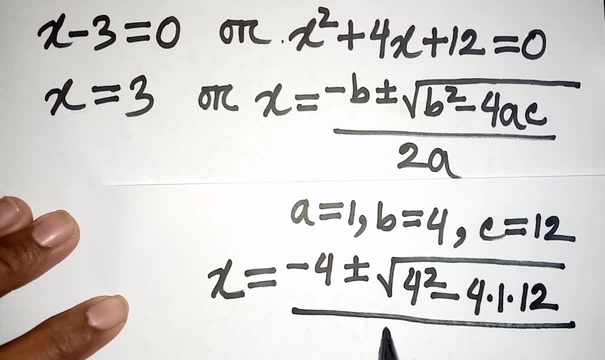 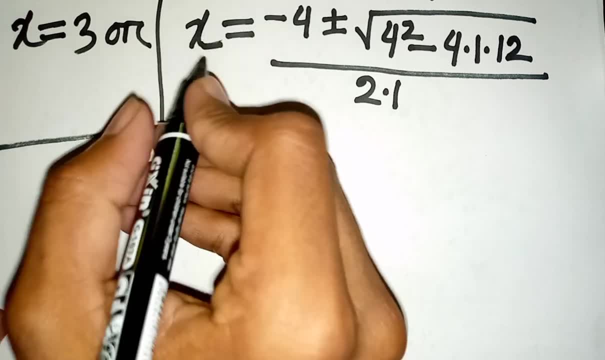 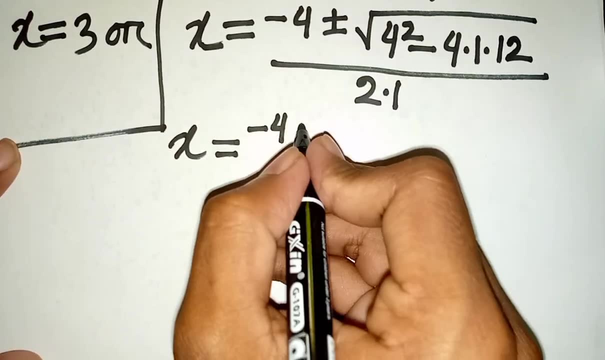 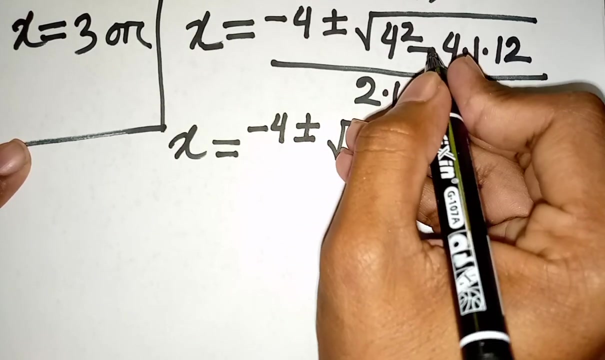 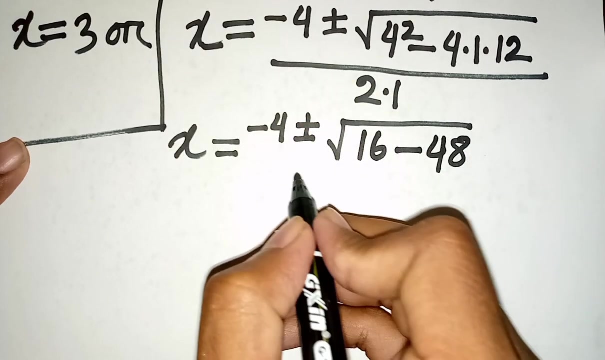 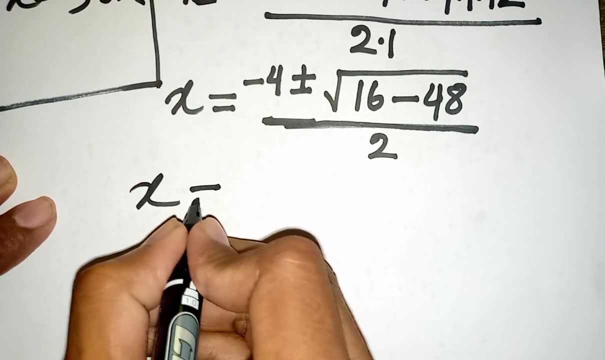 divided by 2 times a, that means 1.. Now we can write here: x is equal to minus 4 plus or minus. a square root of 4 square. that means 16 minus 4 times 1 times 12, that means 48 divided by 2 times 1, that means 2.. Now we can write here: x is equal to minus 4 plus. 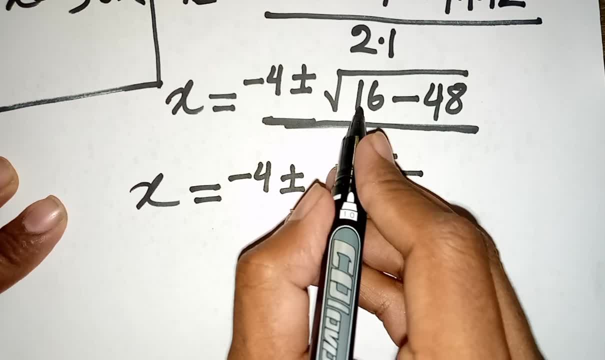 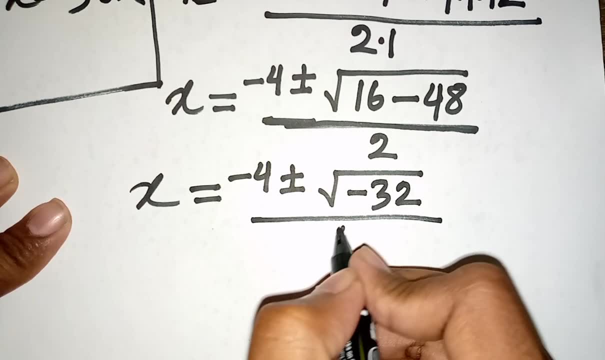 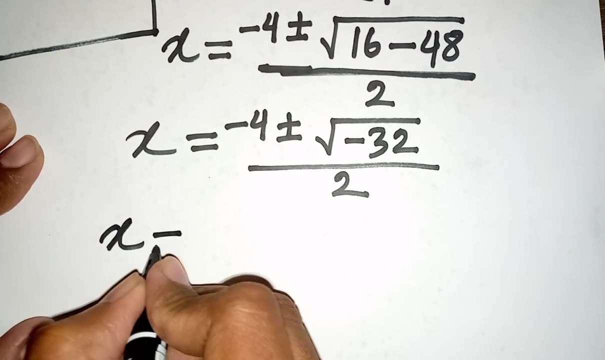 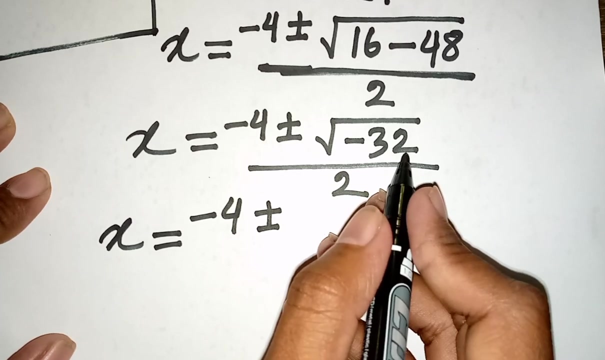 or minus a square root of 16 minus 48, that means minus 32 divided by 2.. Now we can write here: x is equal to minus 4 plus or minus a square root of 16 minus 48, that means minus 2.. Now we can write here: x is equal to minus 4 plus or minus a square root of minus 32. 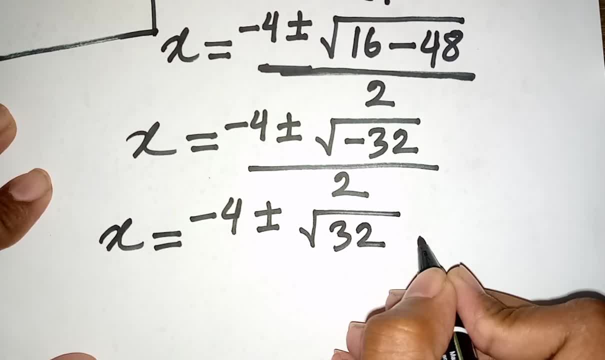 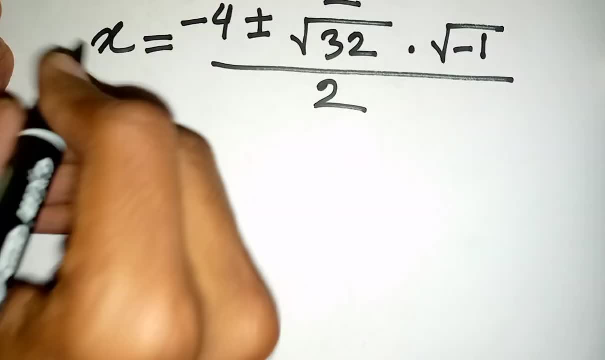 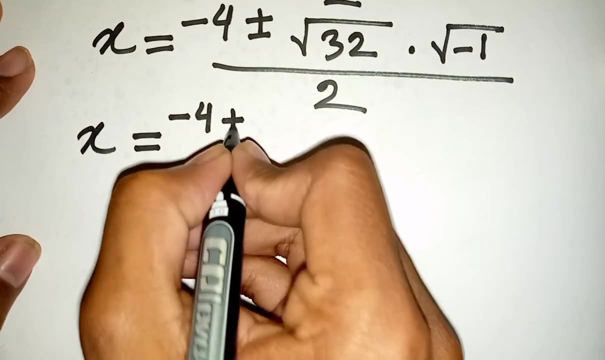 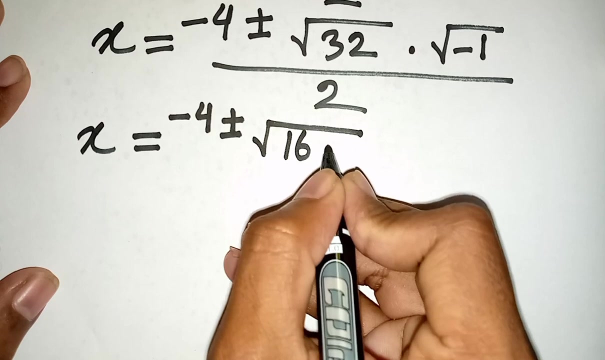 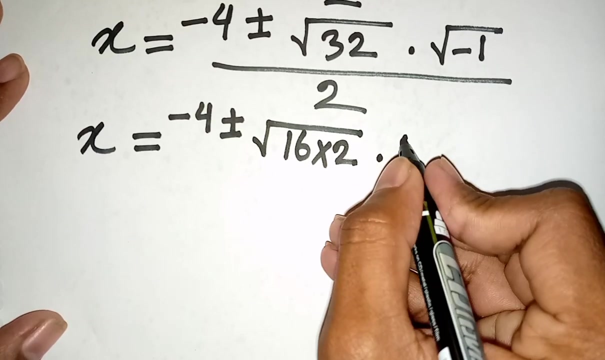 is same as a square root of 32 times a square root of minus 1 divided by 2.. Now we can write here: x is equal to minus 4 plus or minus. a square root of 32 is same as a square root of 16 times 2.. Then, times a square root of minus 1 is same as imaginary divided by 2.. 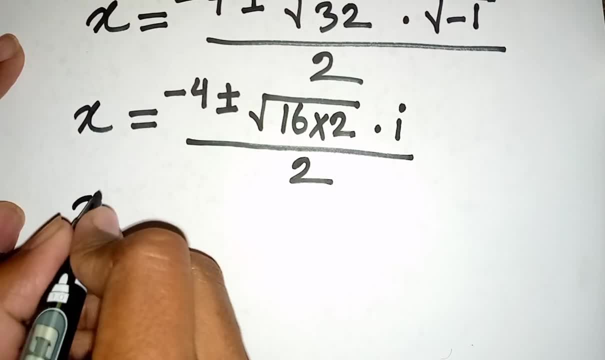 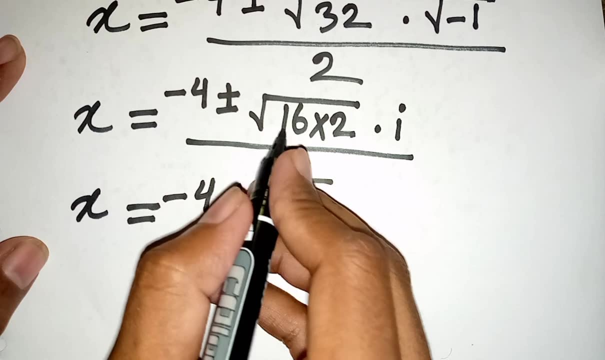 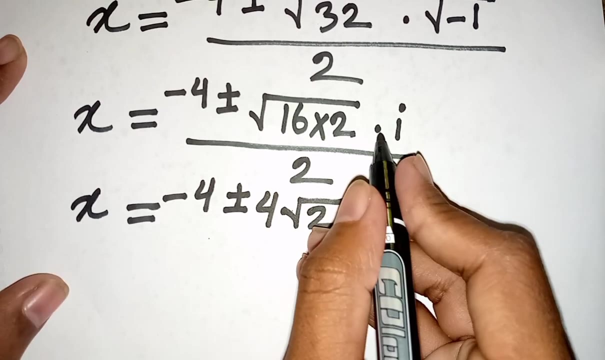 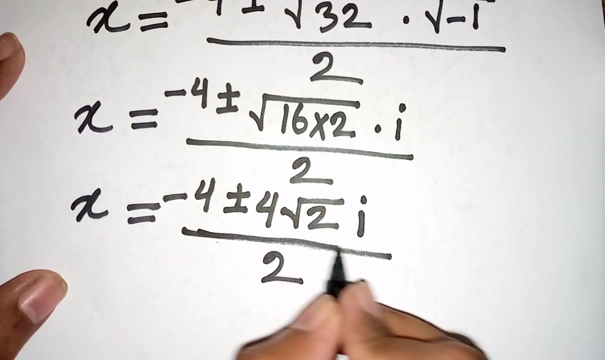 Now we can write here: x is equal to minus 4, plus or minus a square root of 16. that means 4 times a square root of 2, that means a square root of 2.. Then times imaginary, so that means imaginary divided by 2.. Now we see here two cases. so 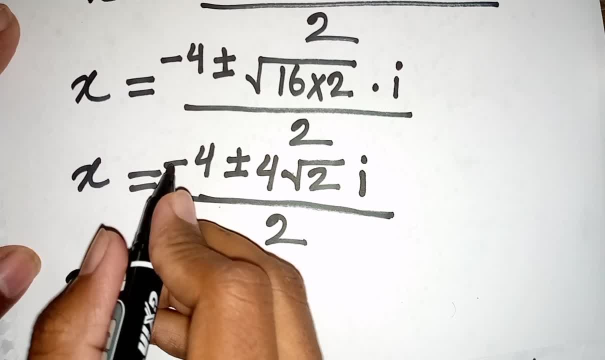 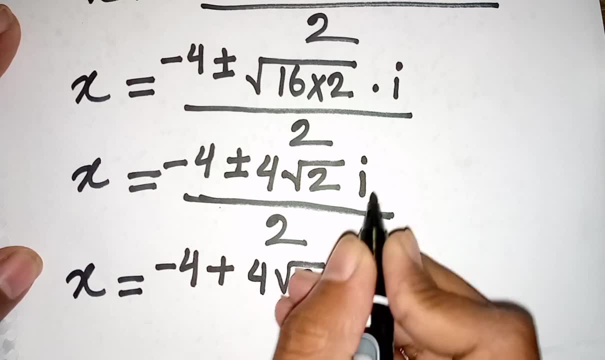 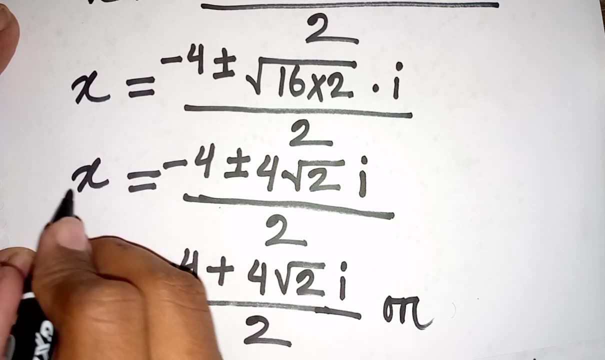 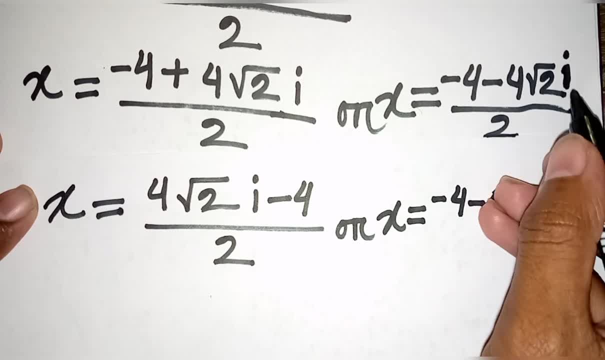 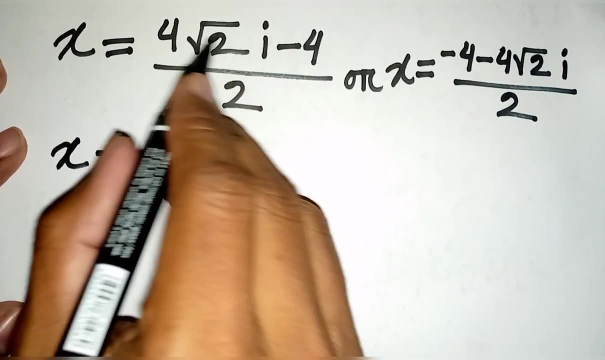 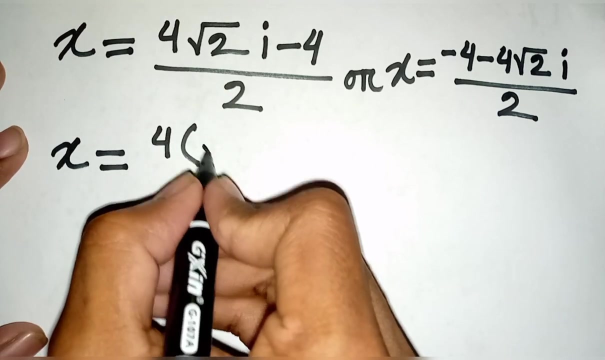 4, square root of 2, imaginary divided by 2, divided by 2.. Now we can write here: x is equal to. we see here: 4 is common, so 4 is out of the bracket. this divided by this, that means square. 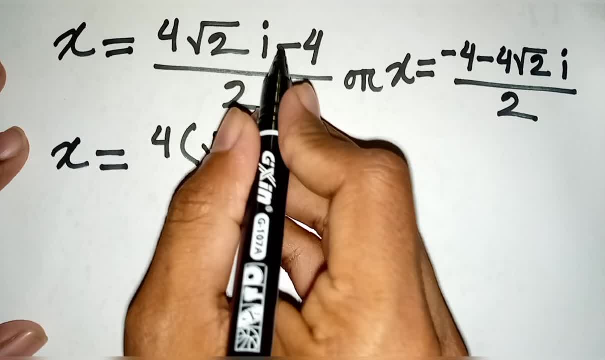 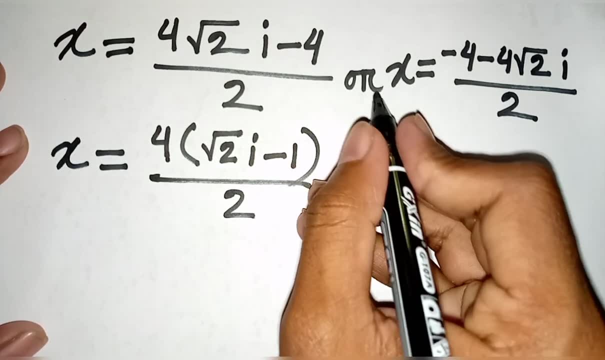 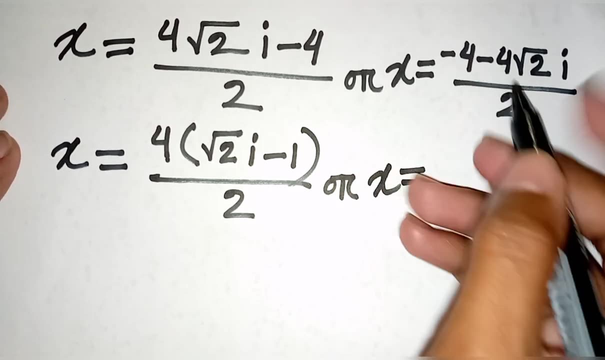 root of 2, imaginary minus. this divided by this, that means 1 divided by 2, or x is equal to. we see here minus 4 is common, so minus 4 is out of the bracket. this divided by this, that means: 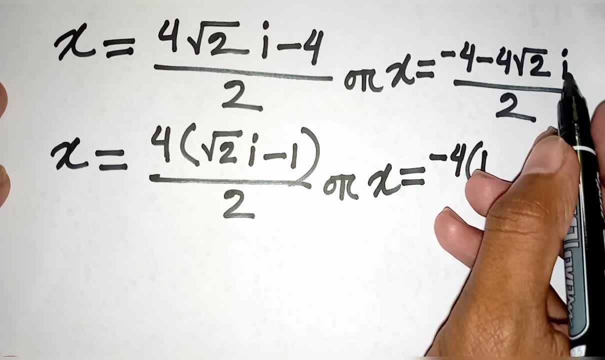 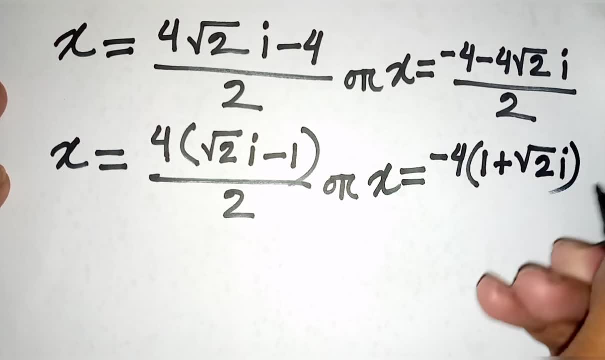 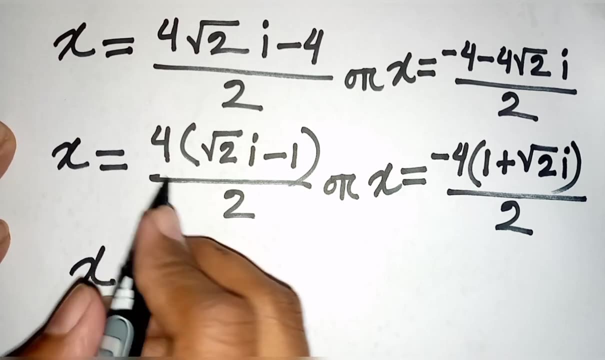 1, then minus 4: square root of 2 imaginary divided by minus 4, that means plus square root of 2 imaginary divided by 2.. Now we can write here: x is equal to 4 divided by 2,. 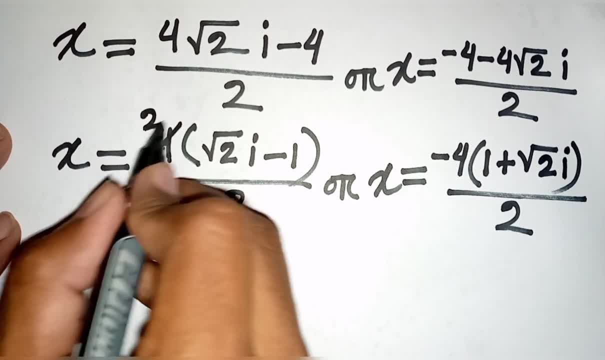 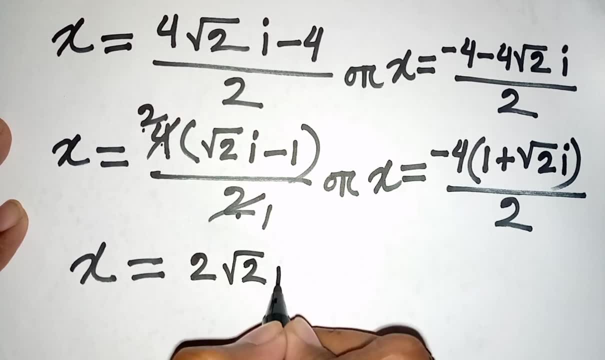 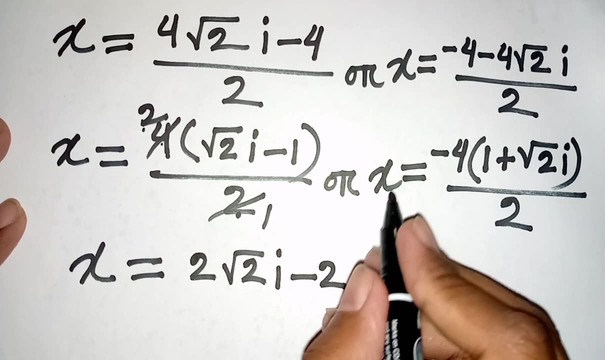 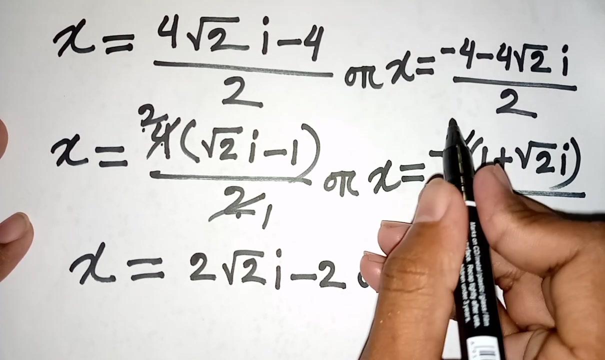 that means 4. simplify by 2,, that means 2, 2. simplify by 2,, that means 1,. 2, square root of 2. imaginary minus 2 times 1,, that means 2,. or we can write here: x is equal to 4. simplify by 2,, that means 2, 2. simplify by 2,, that means 1,. 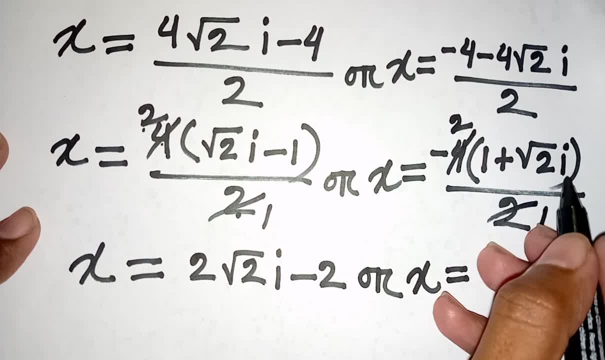 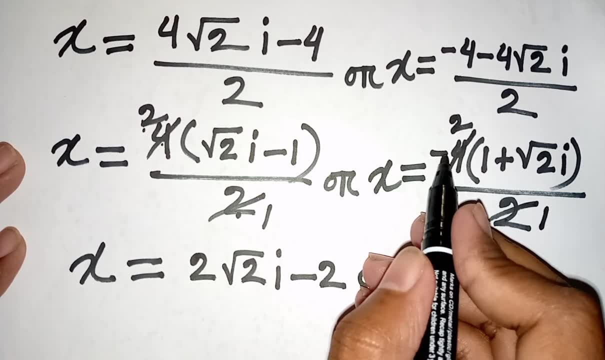 so here: minus 2 times 1 plus square root of 2 imaginary divided by 1, so that means minus 2 times 1, it will be minus 2, then minus 2 times plus square root of 2 imaginary. that means minus.